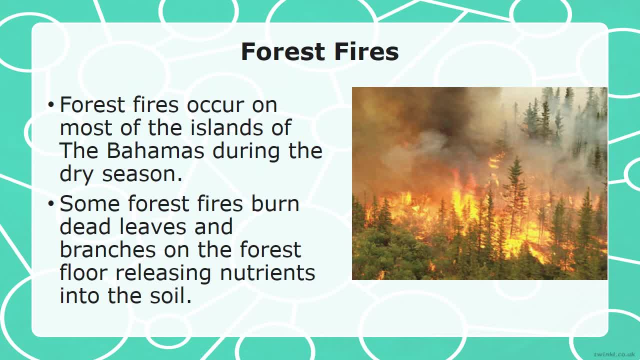 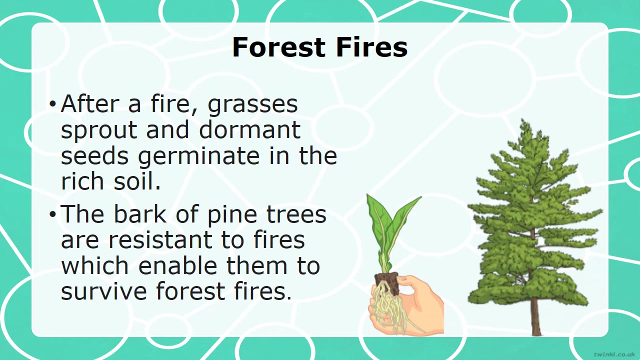 Forest fires. Forest fires occur on most of the islands of the Bahamas during the dry season. Some forest fires burn dead leaves and branches on the forest floor, releasing nutrients into the soil. After a fire, grasses sprout and dormant seeds germinate in the rich soil. The bark of pine trees. 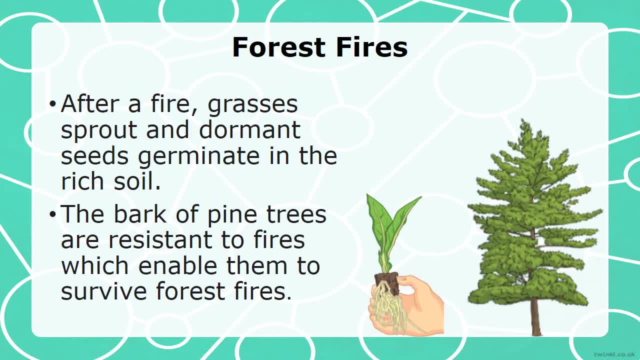 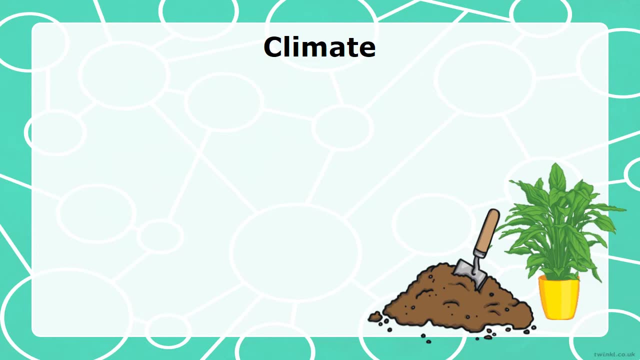 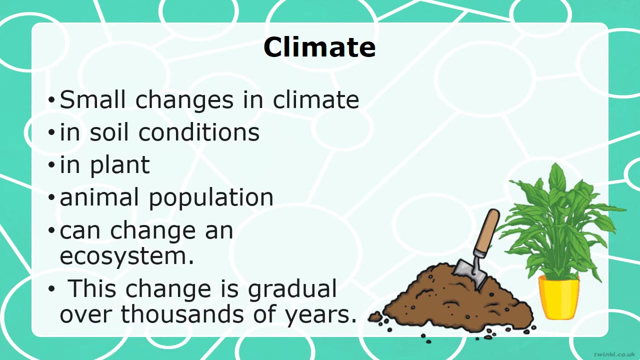 in the Bahamas are resistant to fires, which enable them to survive the forest fires. Let's look at how climate can affect the environment. Small changes in climate can change our soil condition, change our plants, change our animal population and can change our ecosystems totally. These changes are gradual, over thousands of years. 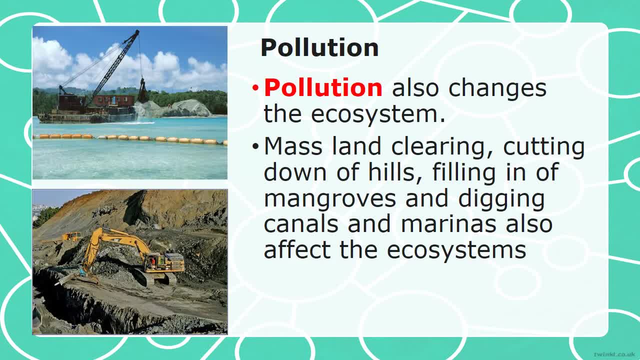 иса Pollution also changes the ecosystem. Mass land clearing, cutting down of hills, filling in of mangroves and digging canals and marines also affect the ecosystems. So the problem of conditions is that in our pickups today we have a population that is. 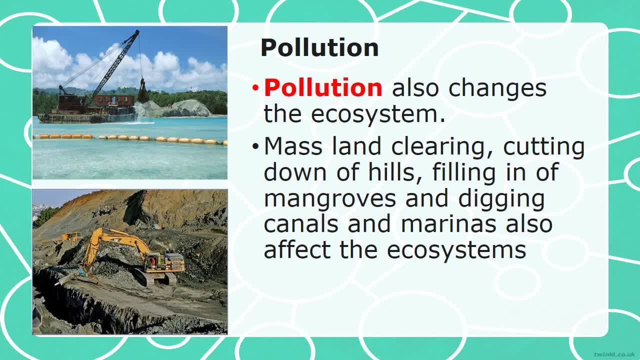 resolved to be 지금까지 polluted. Arknights are especially vital to this. In our These stages, see that the climate is at the transmission level, increasing nutrition consumptions And the inhabitance of the urban industry as per well as the participants, according to點ádé. 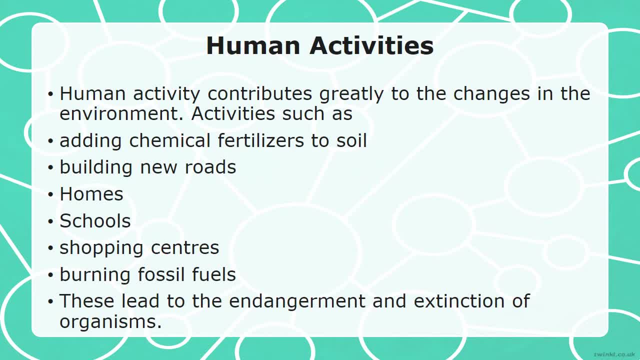 Human Activities. how do they affect our ecosystem? Human activity contributes greatly to the changes in the environment: Activities such as adding chemical fertilizers to the soil, building new roads, building homes, building schools, building shopping centers and also the burning of fossil fuels.